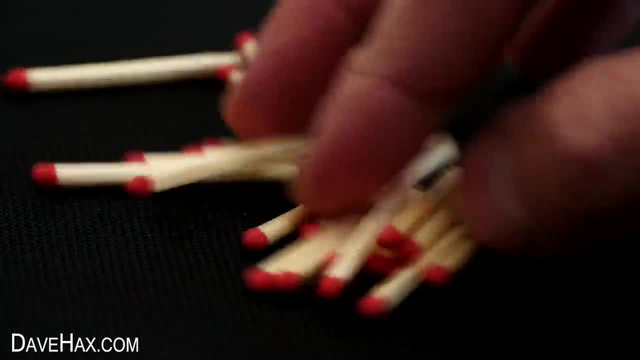 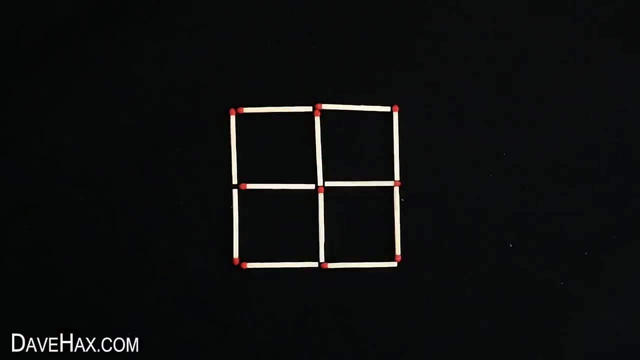 Today I'm going to entertain you with a selection of matchstick puzzles for you to try and solve. For the first one, I've arranged 12 matches like this: Can you create three equal sized squares from this by only moving three matchsticks? The matches must be connecting and you do need to use all the sticks. 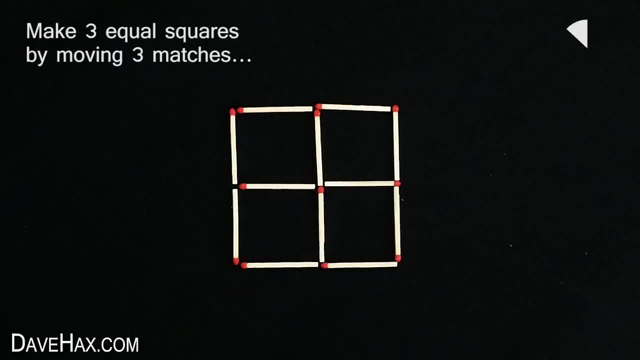 If you want to, you can pause the video to give you more time. Here's how to do it. For the next one, I've arranged the sticks like this: Can you make four equal sized squares by moving only three matches? Here's how. 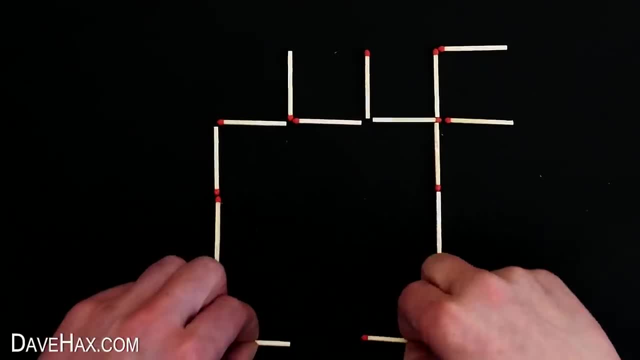 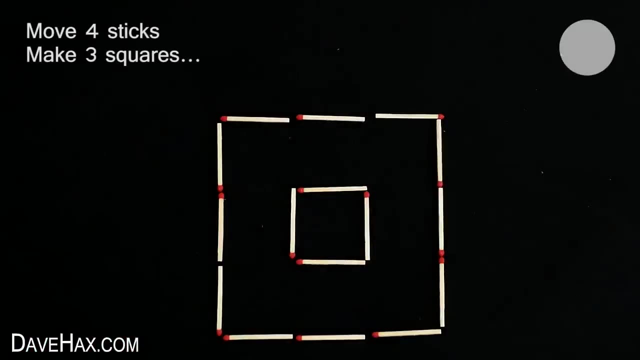 For this one, I'm going to arrange the sticks like this: Can you make a three by three stick square with a one by one square in the middle? Can you move four sticks to make three squares? If you're struggling, here's a clue: The squares don't have to be the same size. 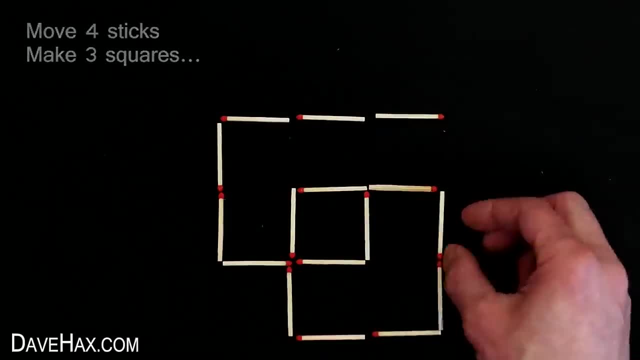 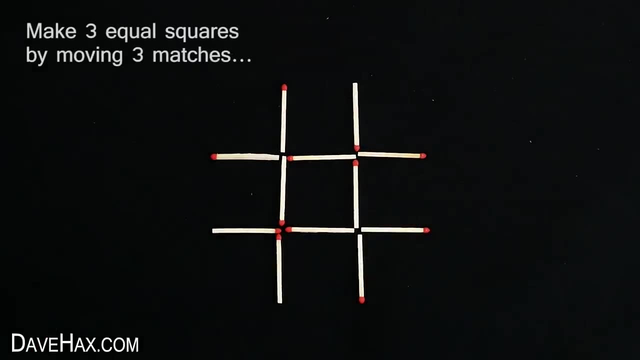 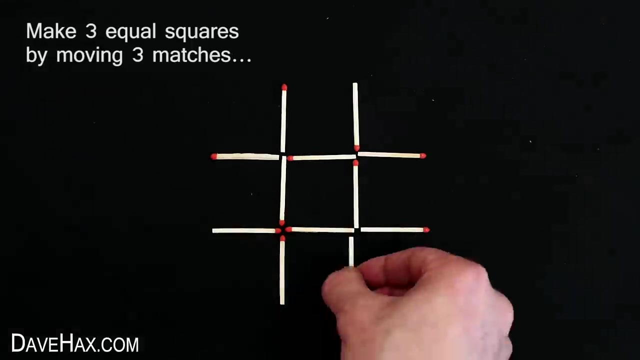 Here's how to do it: Two big squares overlapping with a small square in the middle. Next, I'm arranging the sticks like this And I want to see three equal sized squares by moving three sticks. Here's how It's: the same pattern as the first one we did. 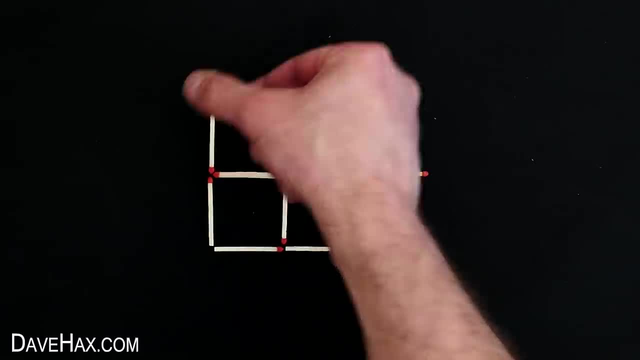 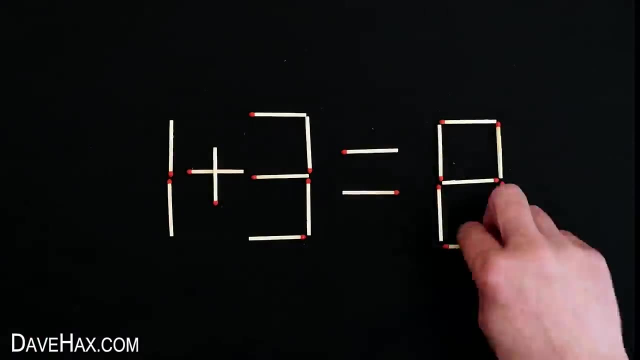 And, if you want to, you can move three sticks again to create our initial starting pattern. The next one I'm arranging is a maths problem. One plus three equals eight. This is obviously incorrect. So can you move two matchsticks to make the equation true? 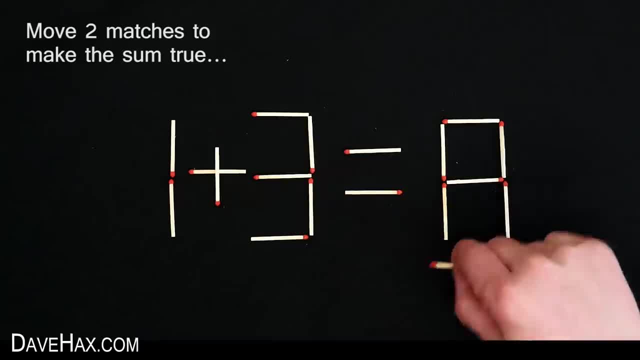 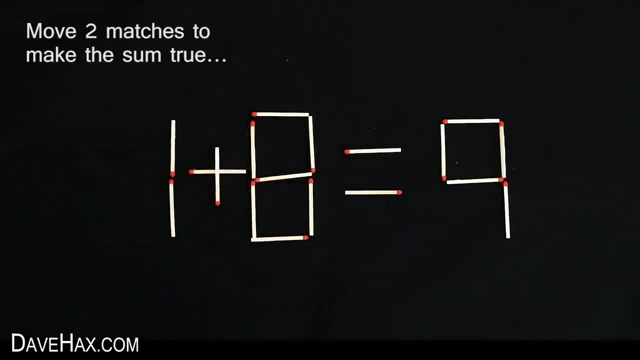 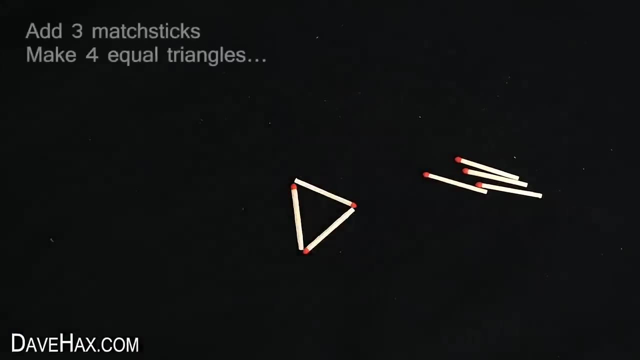 Here's how: If we move the bottom stick from the eight over to this side here And this stick over too, We get one plus eight equals nine. True For the next one. I'm arranging three sticks into a triangle like this. Can you use three more sticks to create four equal sized triangles?